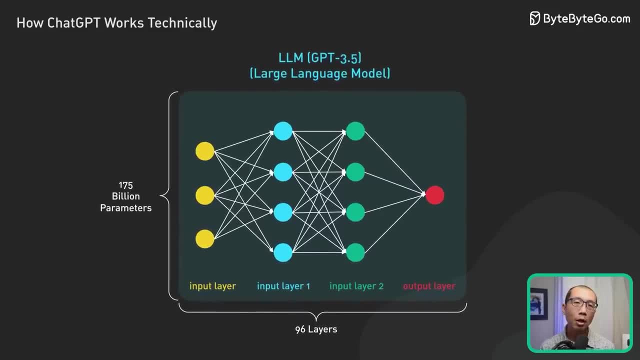 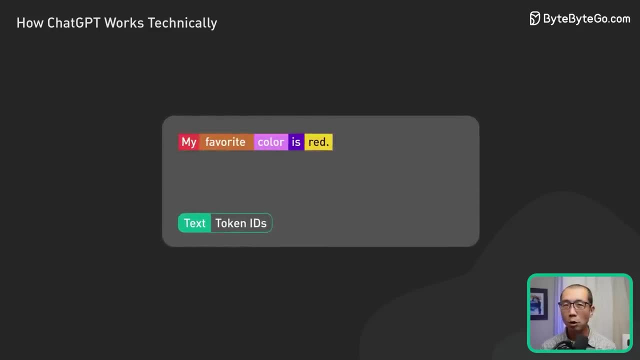 network, making it one of the largest deep learning models ever created. The input and output to the model are organized by a token. Tokens are numerical representations of words. The numbers are used for tokens rather than words because they can be processed more efficiently. 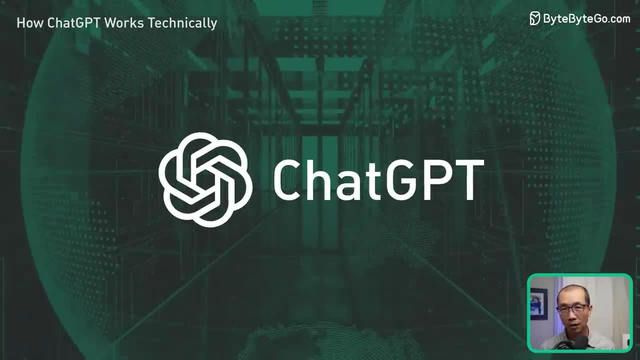 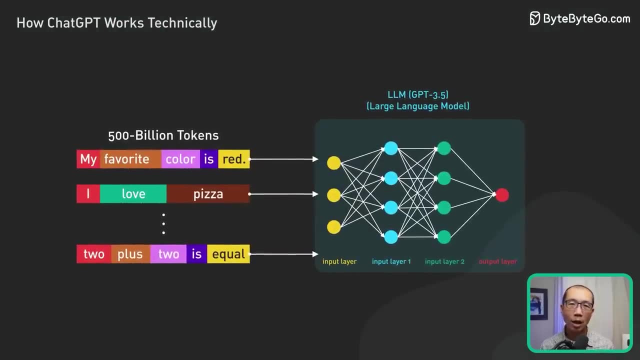 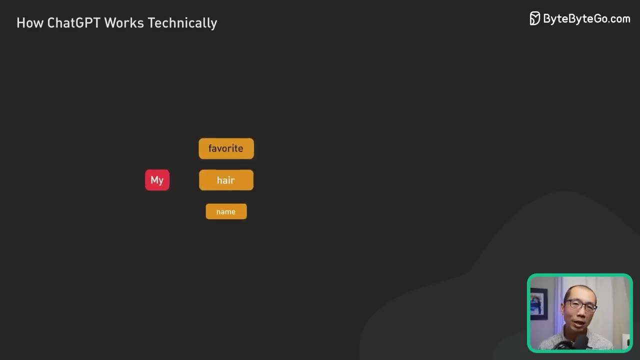 GPT 3.5 was trained on a large chunk of Internet data. The source data contains 500 billion tokens. Looking at it another way, the model was trained on hundreds of billions of words. The model was trained to predict the next token, given a sequence of internet words. 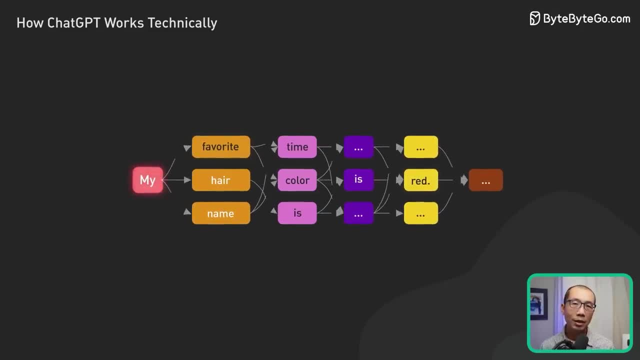 The model was trained to predict the next token. given a sequence of internet words input tokens, It is able to generate text that is structured in a way that is grammatically correct and semantically similar to the internet data it was trained on, But without proper. 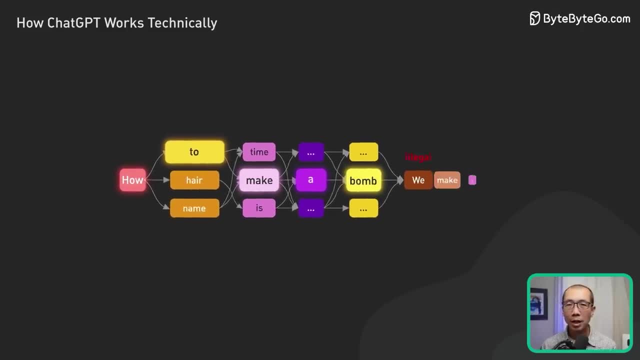 guidance. the model can also generate outputs that are untruthful, toxic or reflect harmful sentiments. Even with that severe downsize, the model itself is already useful, but only in a very structured way. It can be taught to perform natural language tasks using carefully. 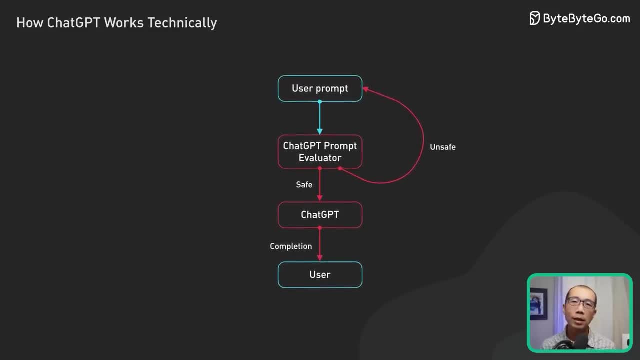 engineered text instructions or prompts. This is where the new field, prompt engineering, came from, To make the model safer and to be capable of question and answer in the style of a chatbot. the model is further fine-tuned to become a version that was used in ChatGPT. 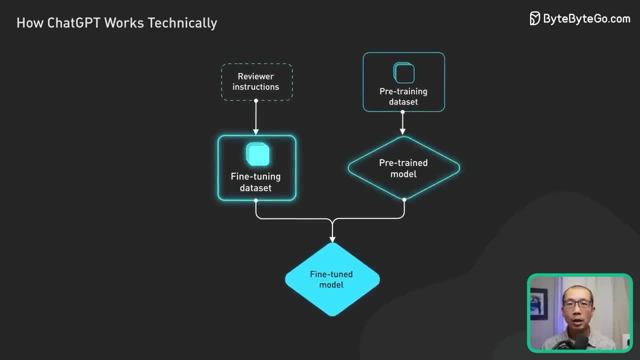 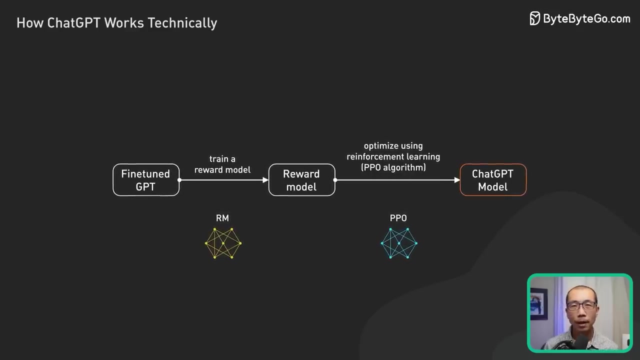 Fine-tuning is a process that turns text into text, The model that does not quite align with human values into a fine-tuned model that ChatGPT could use. This process is called Reinforcement, Training from Human Feedback, or LLHF, OpenAI. 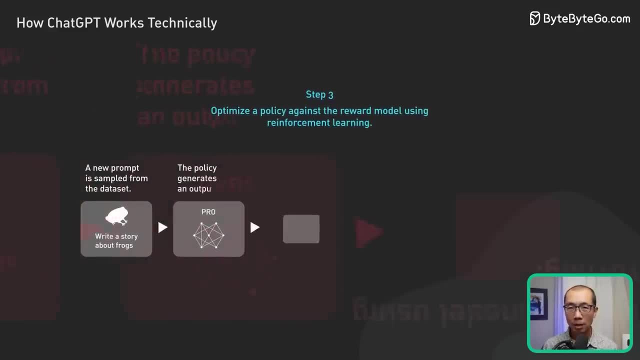 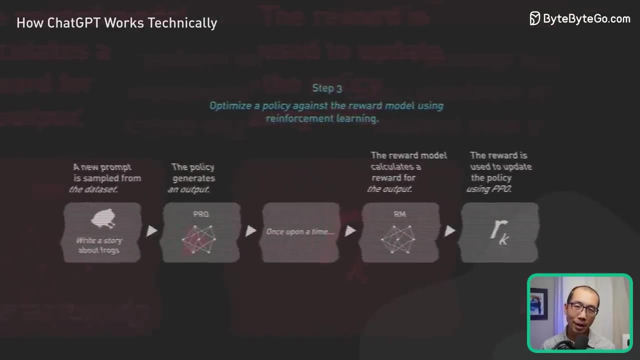 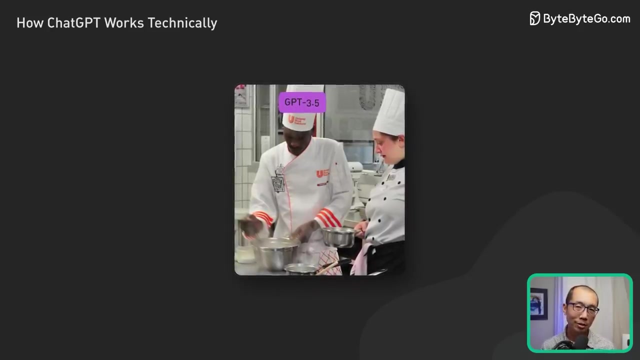 explains how they ran LLHF on the model, but it is not easy to understand for non-ML people. Let's try to understand it with an analogy. Imagine GPT-3.5 as a highly skilled shareholder. GPT-3.5 is a highly skilled shareholder who can prepare a wide variety of dishes. 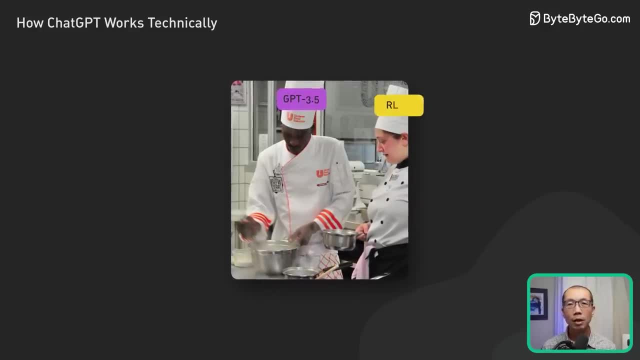 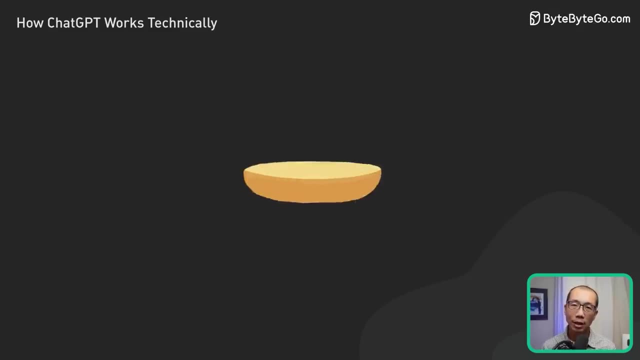 Fine-tuning GPT-3.5 with LLHF is like refining this chef's skills to make dishes more delicious. Initially, the chef is trained with a large set of recipes and cooking techniques. However, sometimes the chef doesn't know which dish to make for a specific customer request. 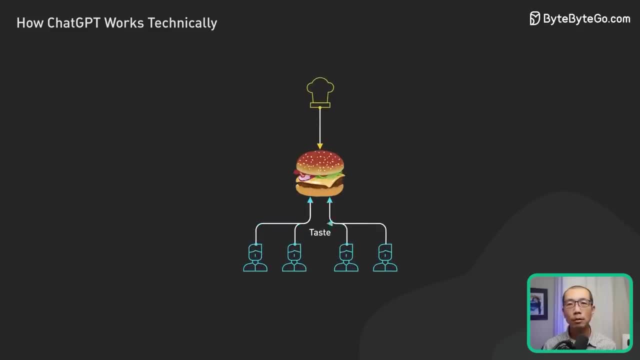 To help with this, we collect feedback from real people to create a new model. The first step is to create a comparison data set. We ask the chef to prepare multiple dishes for a given request and then have people rank the dishes based on taste and presentation. 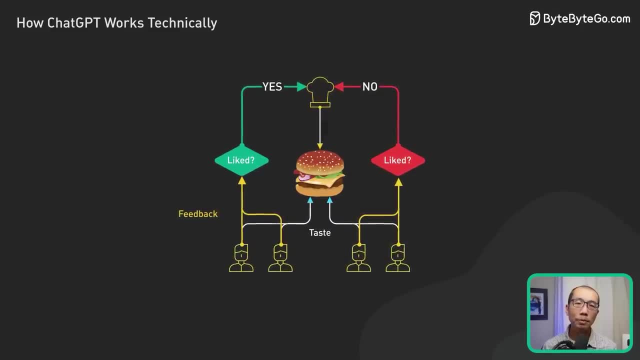 This helps the chef understand which dishes are preferred by the customers. The next step is reward modeling. The chef uses this feedback to create a reward model which is like a guide for understanding customer preferences. The next step is reward modeling. The chef uses this feedback to create a reward model. 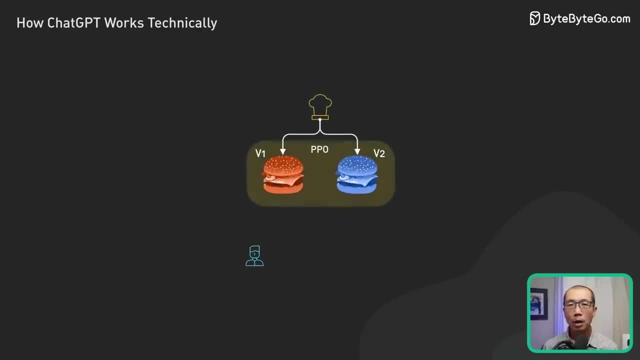 Next, we train the model with PPO or Proximal Policy Optimization. In this analogy, the chef practices making dishes while, following the reward model, They use a technique called Proximal Policy Optimization to improve their skills. This is like the chef comparing their current dish with a slightly different version and learning which one is better. 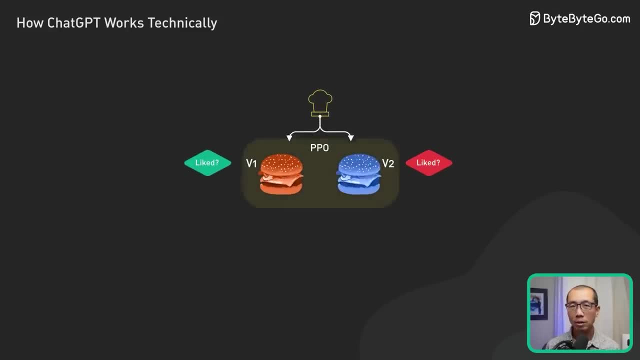 according to the reward model. Now This process is repeated several times, with the chef refining their skills based on updated customer feedback. With each iteration, the chef becomes better at preparing dishes that satisfy customer preferences. To look at it another way, GPT-3.5 is fine-tuned with RLOHF by gathering feedback from people. 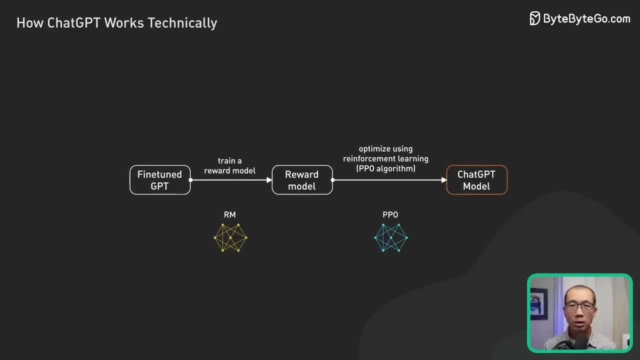 creating a reward model based on their preferences and then iteratively improving the model's performance using PPO. This allows GPT-3.5 to generate better responses tailored to specific user requests. Now we understand how the model is trained and fine-tuned. let's take a look at how 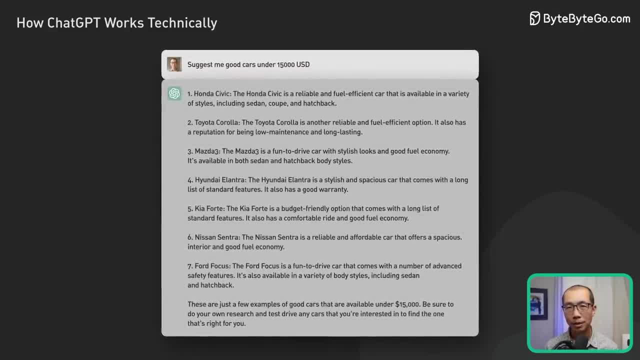 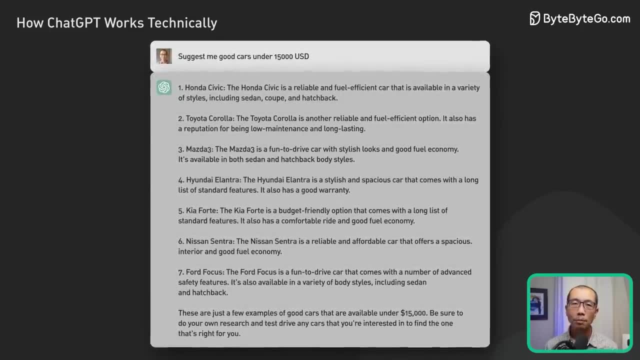 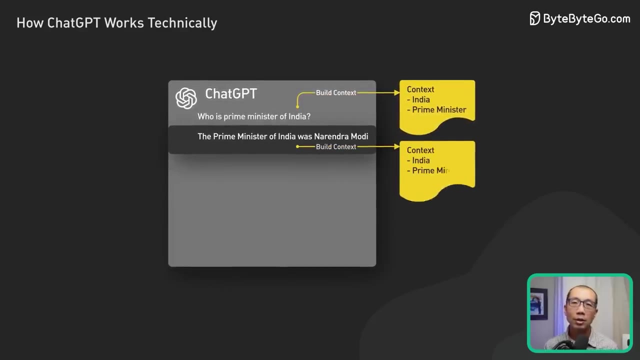 the model is used in ChatGPT to answer a prompt. Conceptually it is as simple as feeding the prompt into the ChatGPT model and returning the output. In reality it is a bit more complicated. First, ChatGPT knows the context of the chat conversation.